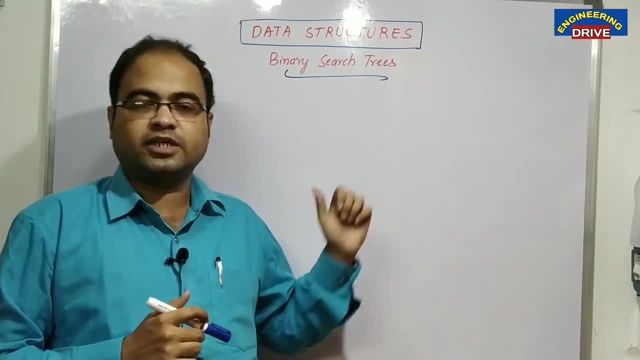 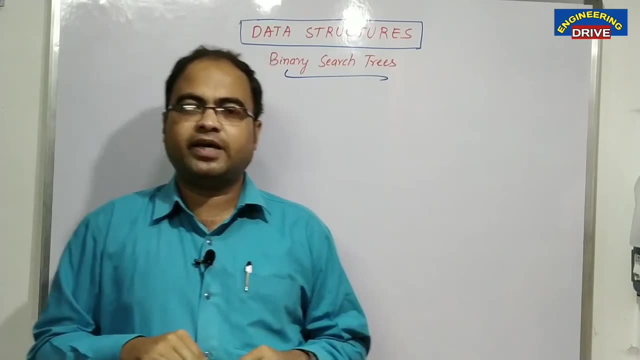 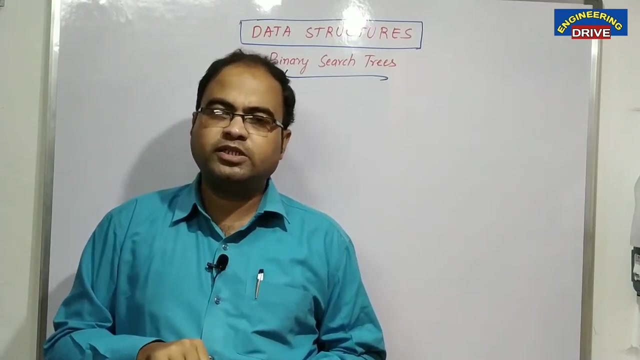 Ok, so let me tell you what is a binary search tree now. So a binary search tree is also a binary tree. You know that. what is a binary tree? In binary tree, a parent will have at most two children. How many children? At most two, Which means 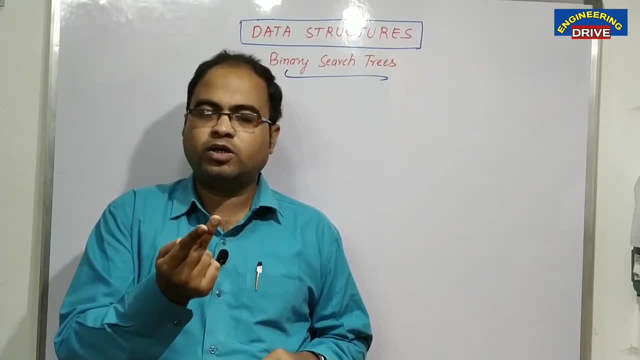 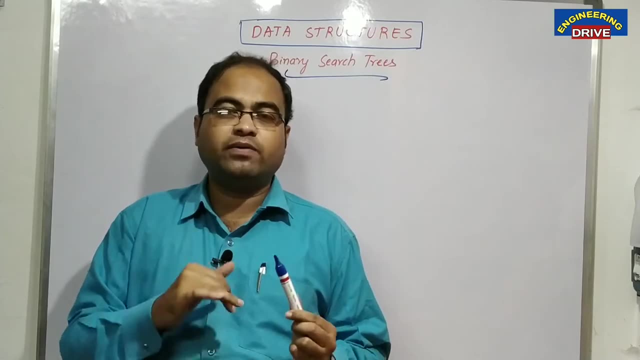 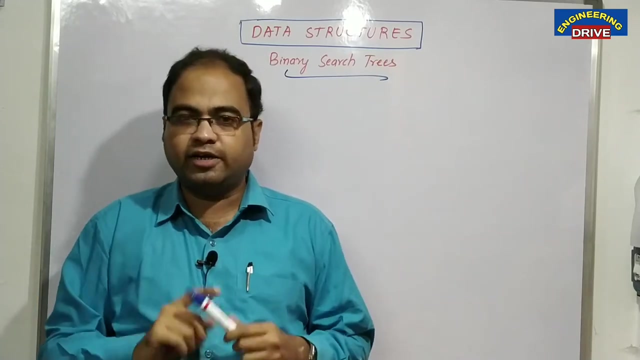 a parent can have zero child node, one child node or two child nodes. A parent node should not have more than two child nodes. If it is having more than two child nodes, it is not a binary tree. Ok, so a binary search tree is also a binary tree, with one specific condition: What is? 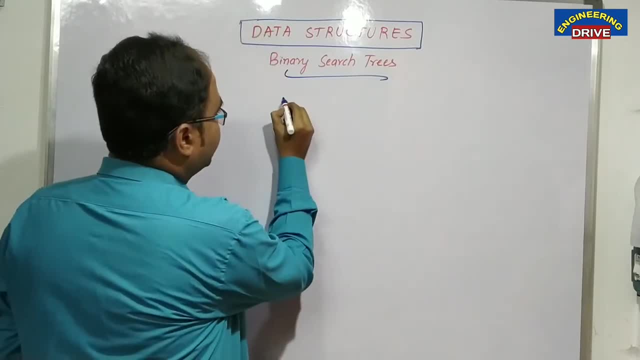 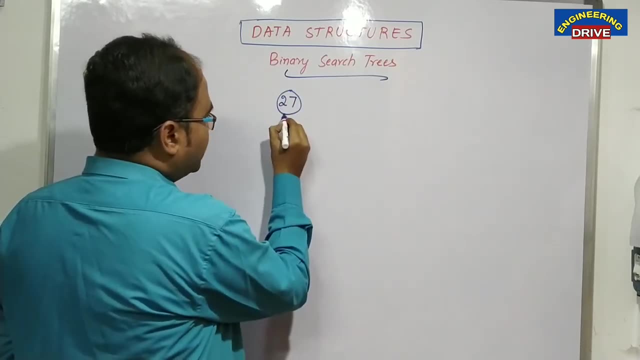 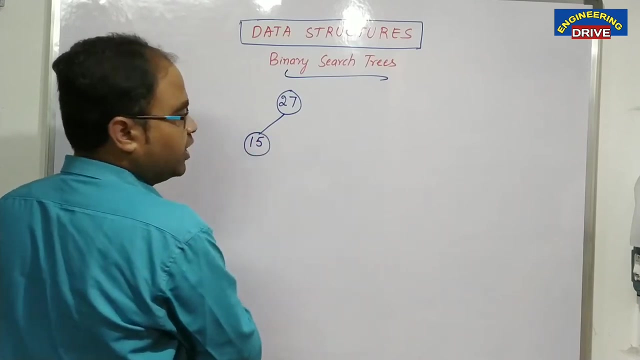 that specific condition means. Let me give you an idea. Let us take 27 as the first root node. Ok, now for this root node. what I am doing here? I am writing one number. Let us say second child, one child, node 15.. 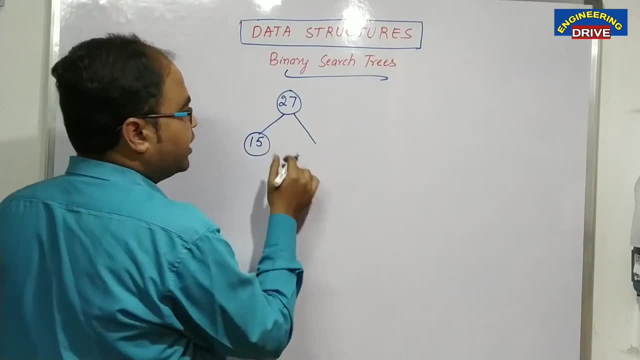 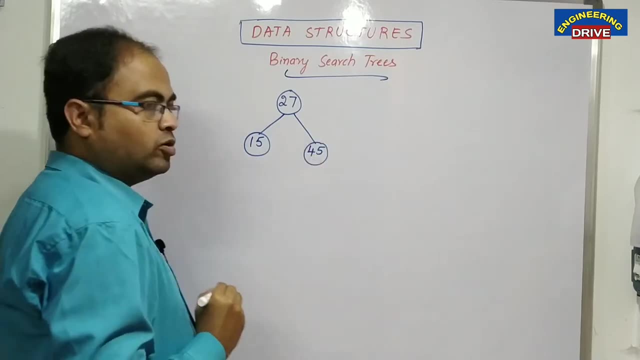 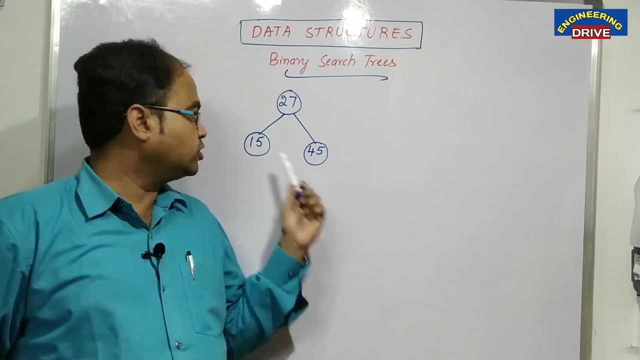 Here for this same root node. what I am doing, I am writing one more value here, Let us say 45. Now you got one clear idea that here we are having one root node. How many child nodes are there here? Two child nodes: One is 15, another one is 45. Whether it is a binary, 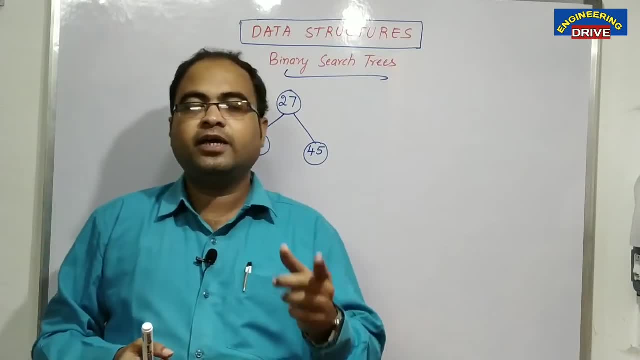 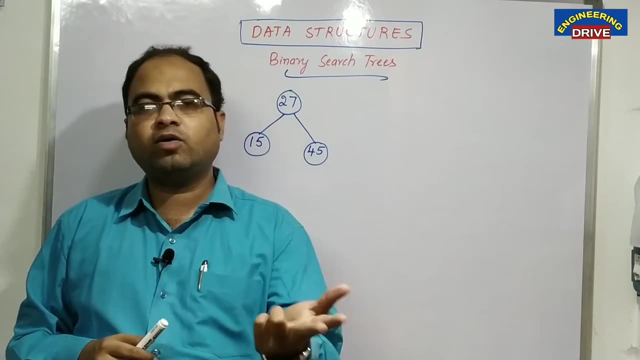 tree? Yes, of course it is a binary tree, Because in binary tree a node can have maximum. how many child nodes? Two child nodes. It can have zero child nodes. How many child nodes? Eight child nodes It can have zero. it can have one or it can have two child nodes. 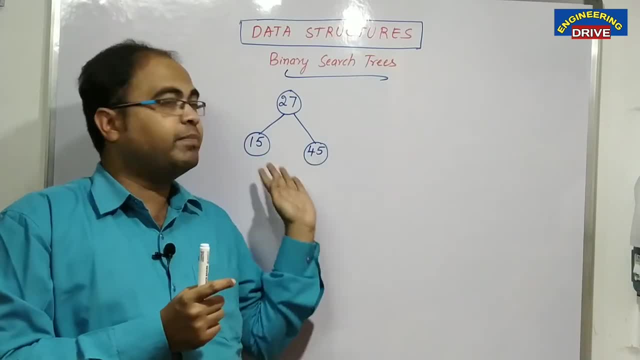 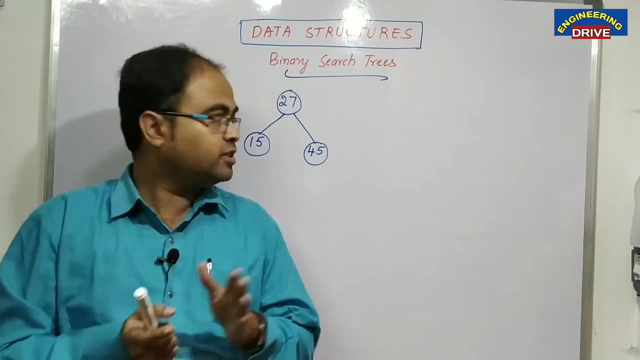 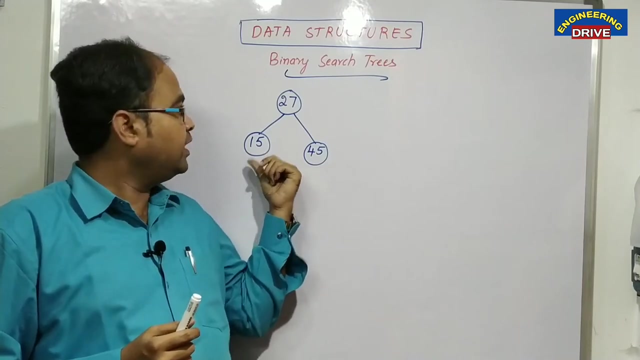 So it is a binary tree. Now, whether it is a binary search tree, Because our topic is binary search tree- A binary search tree is a tree in which the value of left child must be less than the parent And the value of right child must be greater than the parent. 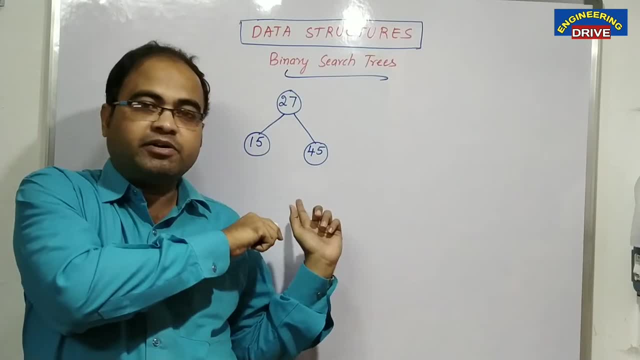 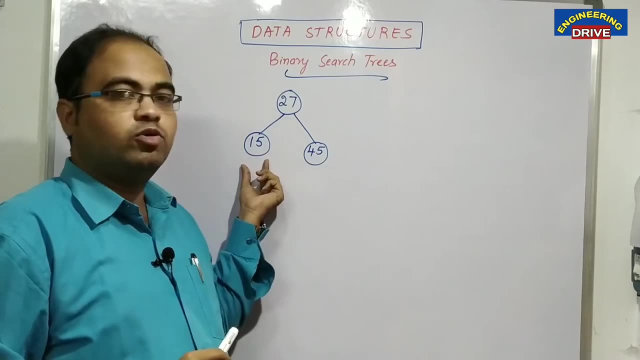 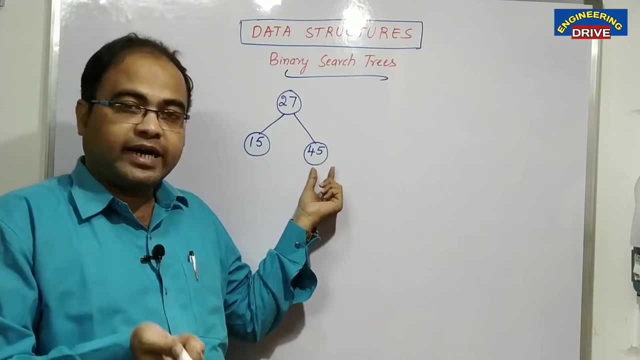 If this condition satisfies, Ok, that binary tree becomes a binary search tree. Now let us see whether this condition is satisfied or not. here Left child node value, whether it is smaller than parent or root node. Yes, it is smaller, Okay. Next condition: whether- right- child value is greater than the root node. 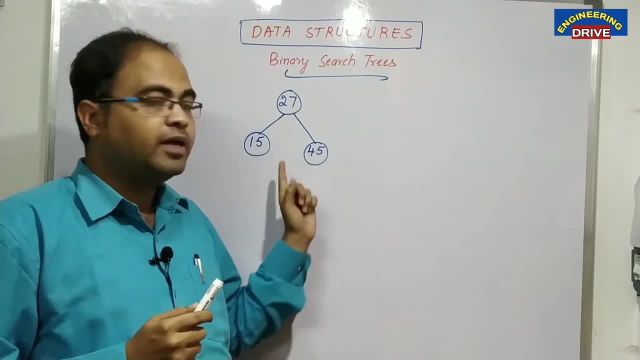 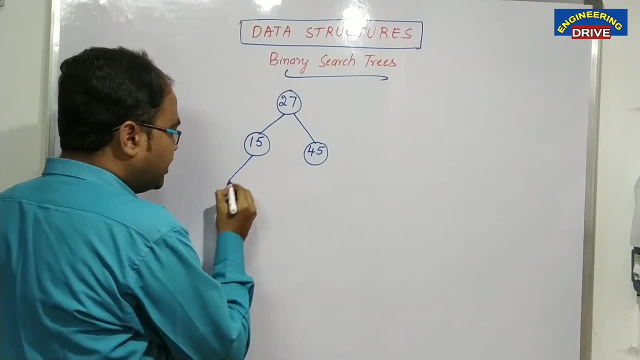 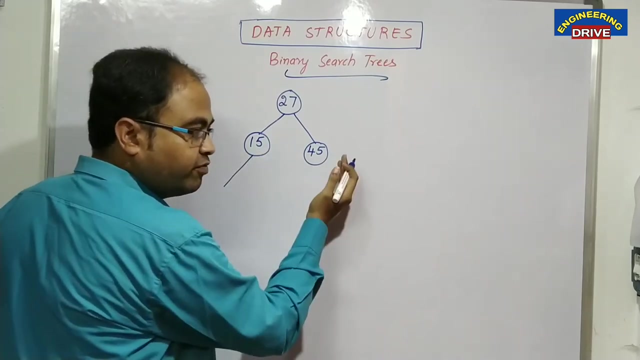 or parent node. Yes, it is also satisfied. So this is a binary search tree. Now, if I want to continue constructing this binary search tree, what I need to do here? Let us take 15 as a parent node Now, whether I should write a number which is less than 15 here or greater than 15?. 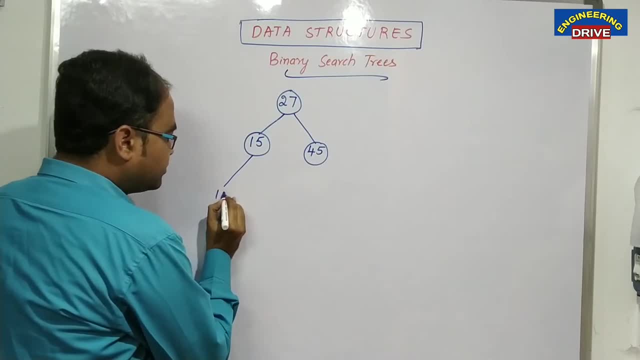 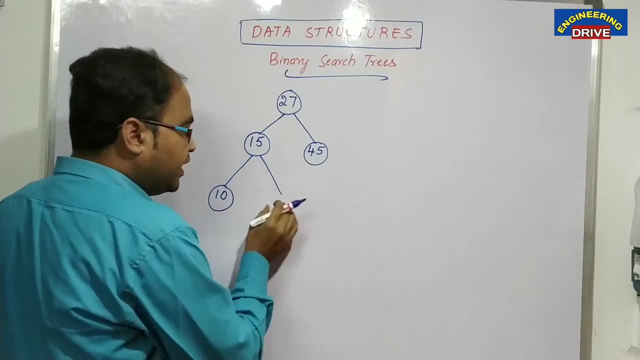 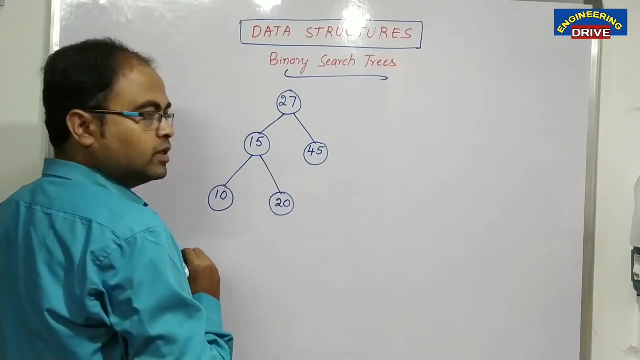 Less than 15.. So here I can write 10.. No problem. Okay, What about this child node? now? Here I should write the value which is greater than 15.. So which means I can write here anything like 20.. Whether still it is a binary search tree? Yes, still it is a binary search tree because 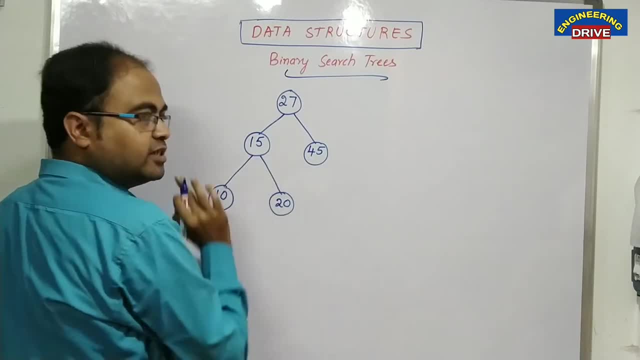 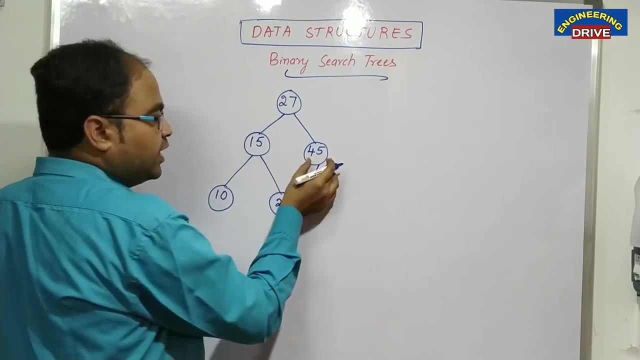 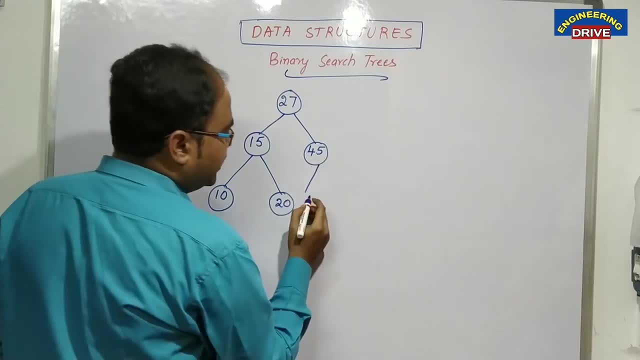 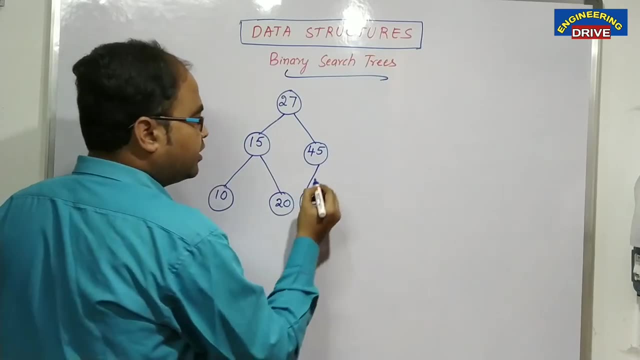 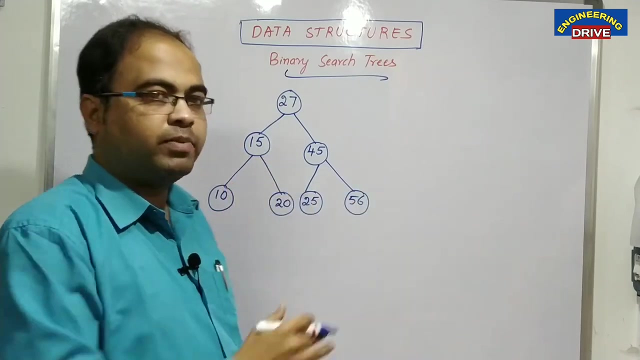 less than 45. So here I can write, let us say 25.. Here I can write, let us say 56.. Now you need to completely go through and tell me whether it is a binary search tree or not. 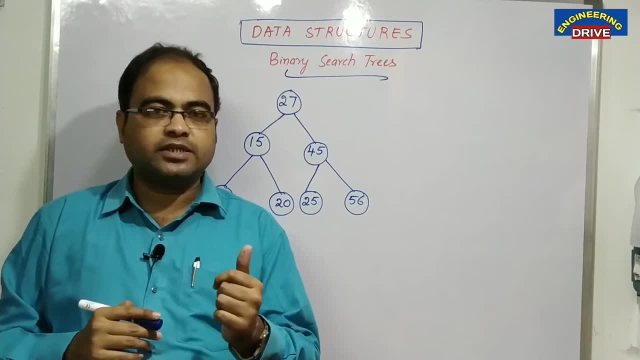 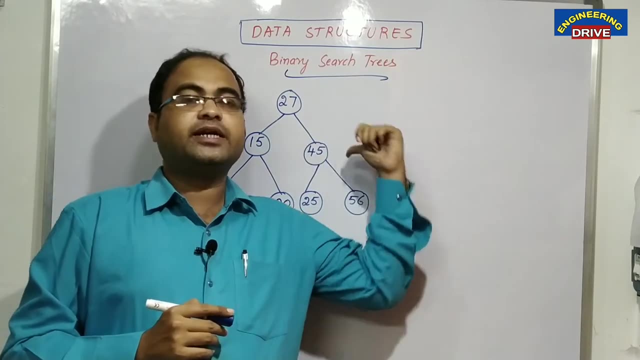 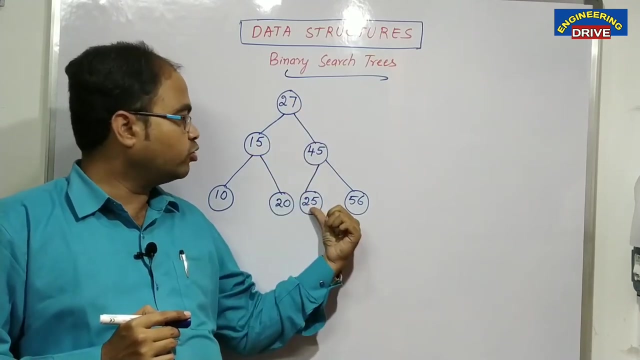 So, first of all, you should know this condition: that in binary search tree the left child value must be less than the parent and the right child value must be greater than the parent: 15 less, 45 greater, 10 less, 20 greater, 25 less, 56 greater. Yes, it is a. 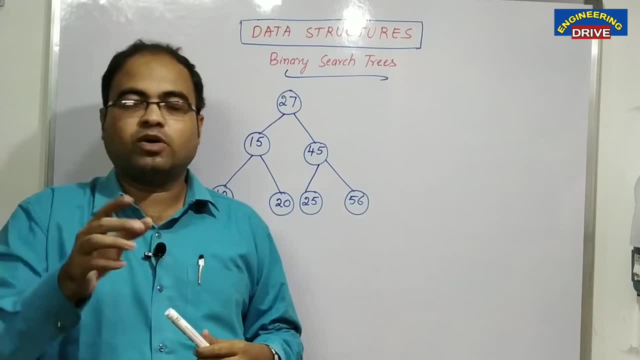 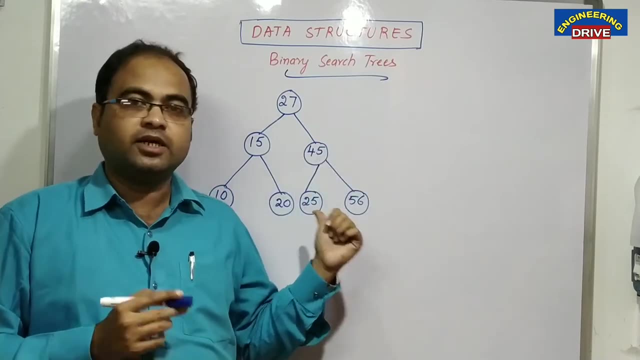 binary search tree. Okay, So sometimes how they will ask the questions in exam they will give which of the following is not a binary search tree. So you need to see the simple condition, Sometimes what they will do here: 45.. So, instead of number, 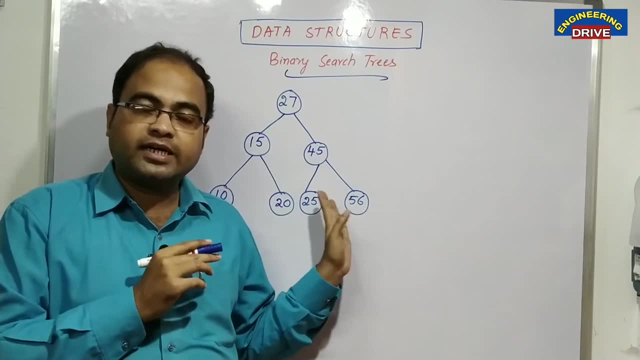 greater than 45, what they will do? 44, they will give here. So at that time, whether it is a binary search tree, it is not a binary search tree. Yes, it is a binary tree, but it is not a binary search. 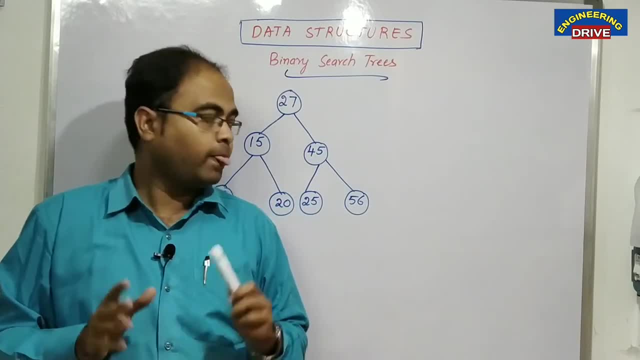 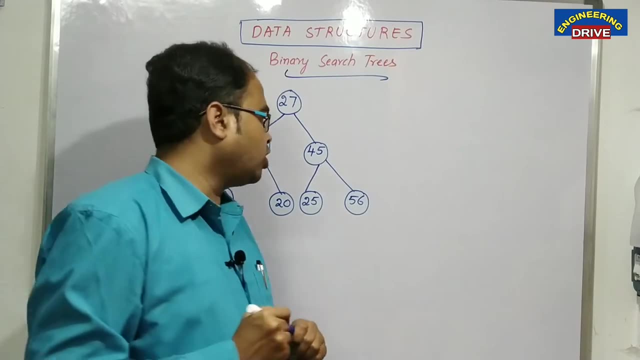 tree, So those type of questions can be asked in competitive exams. Now the next thing, sir, this is a binary search tree. What are the operations we can perform on this binary search tree? There are numerous operations you can perform on a binary search tree, such as: 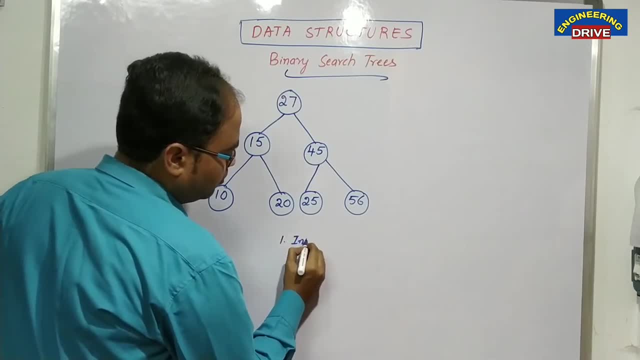 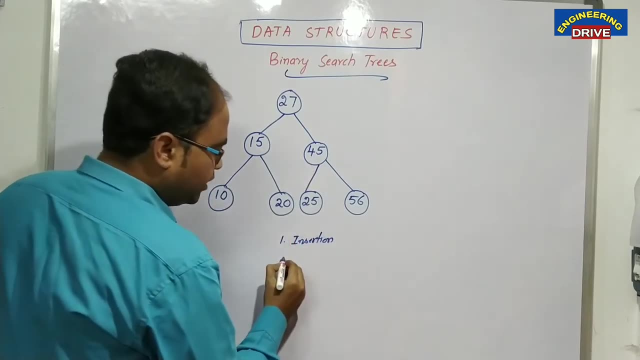 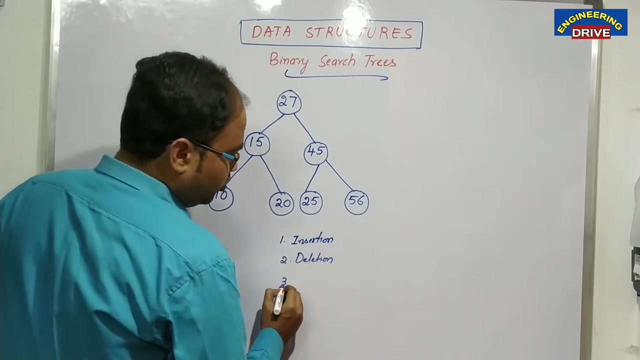 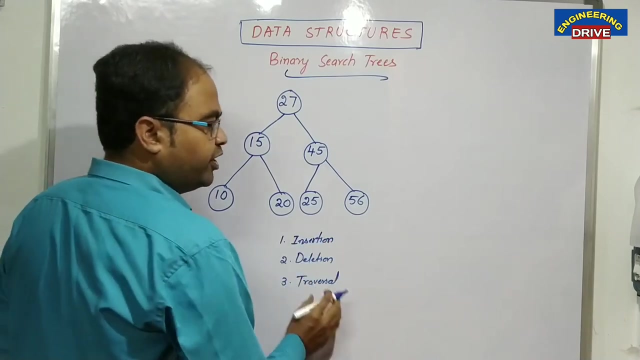 you can perform insertion of the data, which means if you want to insert the notes, you can insert the notes in binary search tree. If you want, you can perform deletion of the notes in binary search tree and you can perform travel cell. What is the meaning of travel cell? You know this is very. 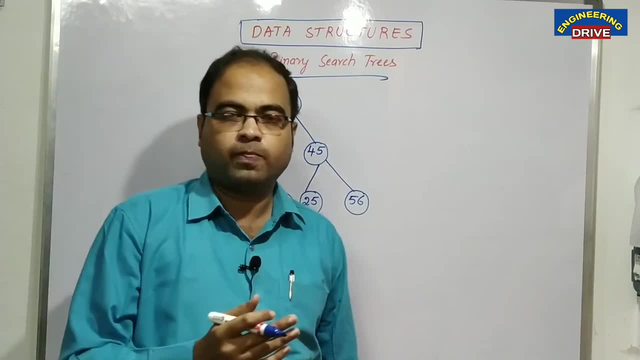 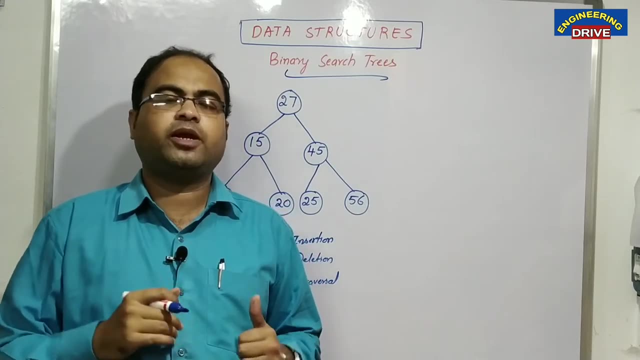 very important topic And surely after some videos once we will complete the various series, I am going to focus on this. travel cell techniques- Very, very important concept and numerous questions has been appeared from this concept. So what are the three travel cell? 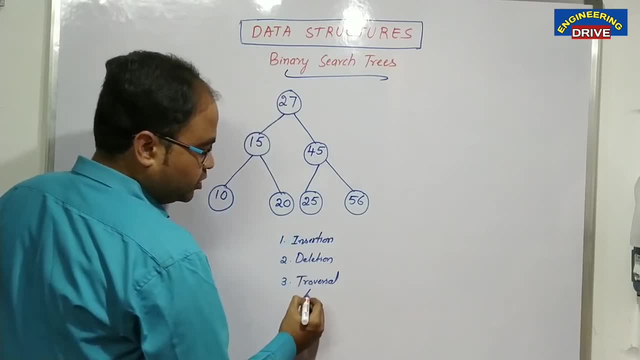 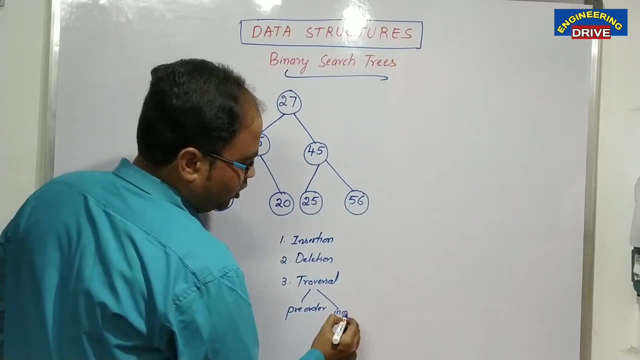 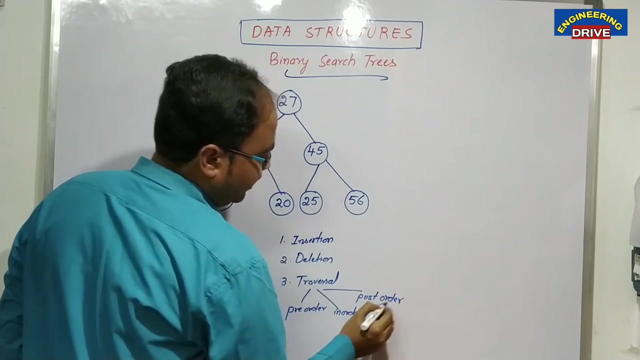 techniques that are available in a binary search tree. So, which means pre-order travel cell? Next, we are having in-order travel cell and we are having one more post-order travel cell, So you can travel. You know what is the meaning of travel cell. 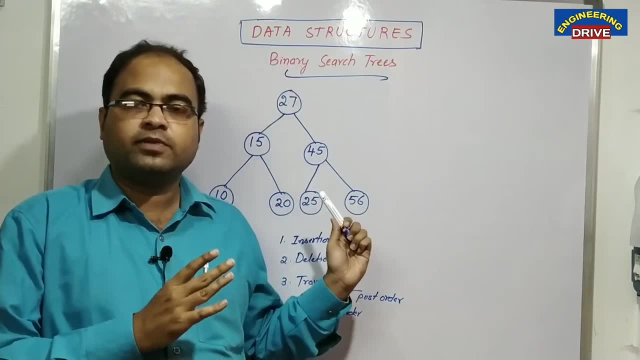 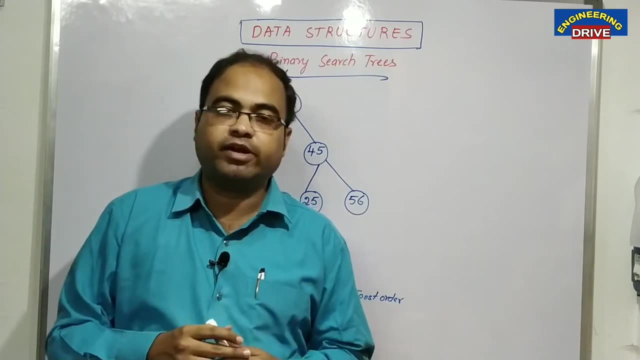 Traversing is nothing but visiting all the nodes of a tree, Visiting one by one node of a tree. If we visit the nodes in a binary search tree, we can call those methods as traversing a tree. And you can traverse a tree in three ways. One is by using pre-order method, in-order method and 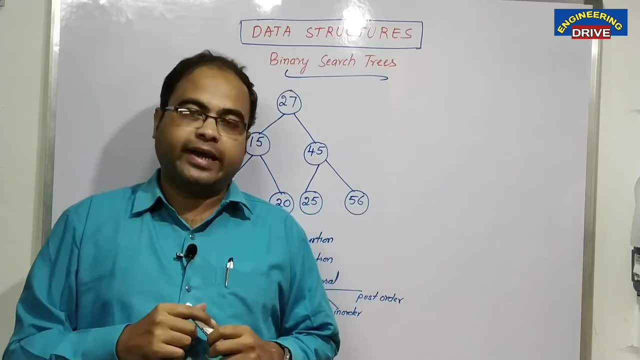 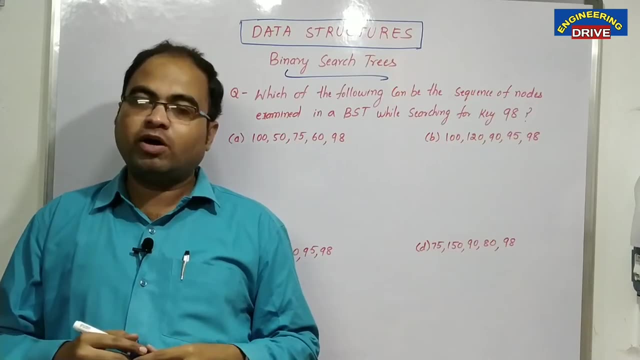 post-order method. So how they will work, you will come to know in our next parts. These are some of the operations that can be performed on a binary search tree. Okay, now I have written one question, one basic question. So what is the meaning of travel cell? So what is the meaning of travel? 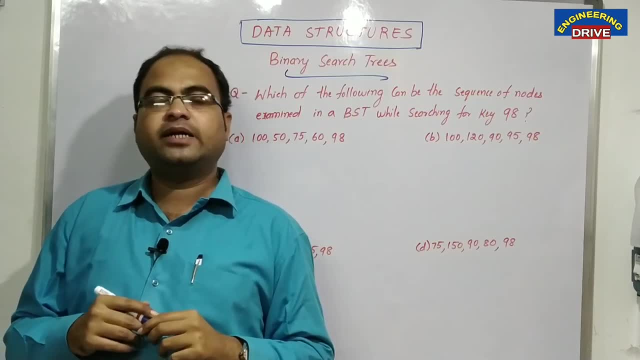 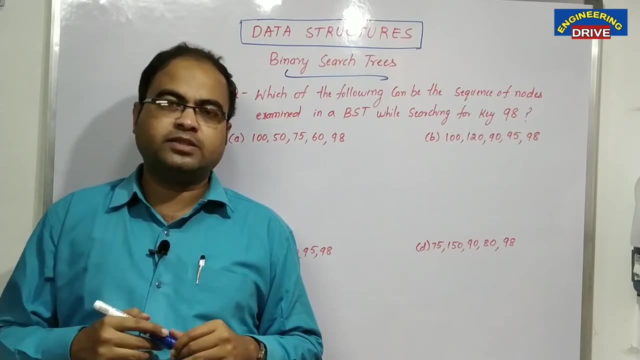 cell. This is a basic question that can come in binary search tree topic and it has been asked in various competitive exams- You can take the example of net set or slit- or even in many companies. This question has been asked in the form of aptitude related problems. So how we can. 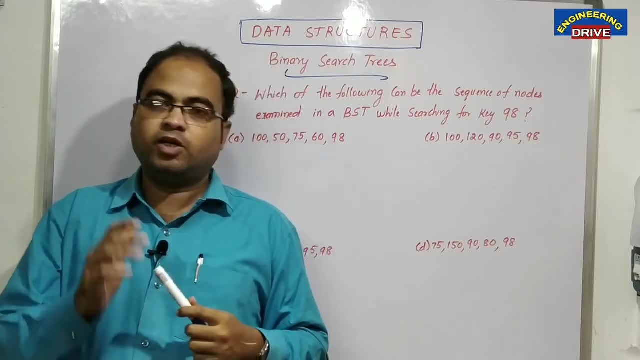 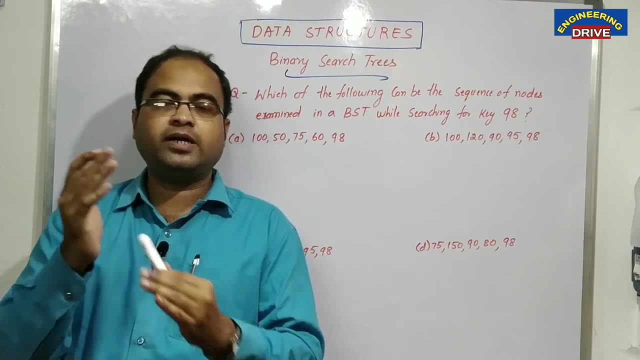 solve this question Now. you have understood what is a binary search tree. You have understood the condition that can be used in a binary search tree, which means the value of left child must be smaller than the parent and the value of right child must be greater than the parent. 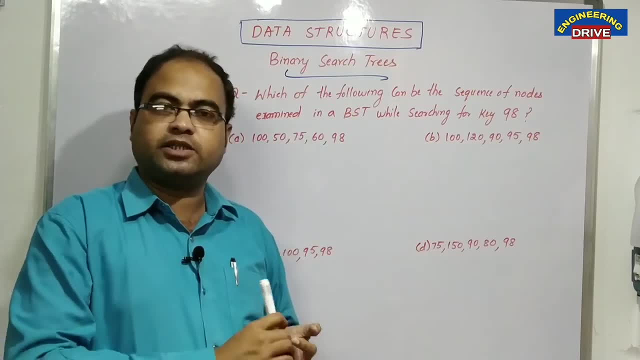 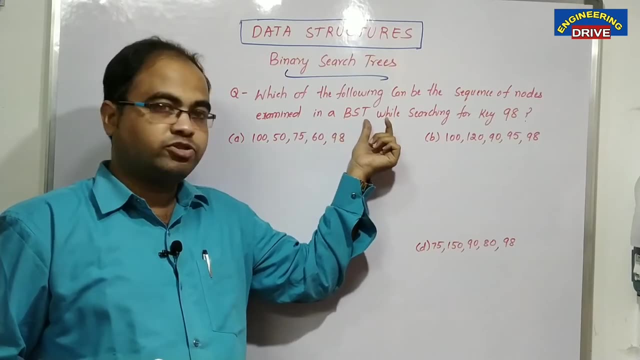 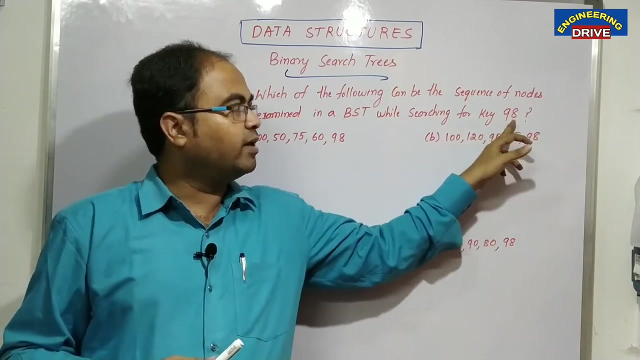 Now there is one question that has been most frequently asked in binary search tree topic, that is, which of the following can be the sequence of nodes examined in a binary search tree while searching for key 98?? So here key refers to one node. I want to search a number. I want to search. 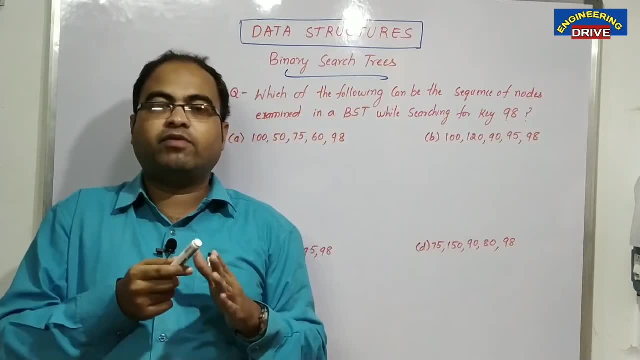 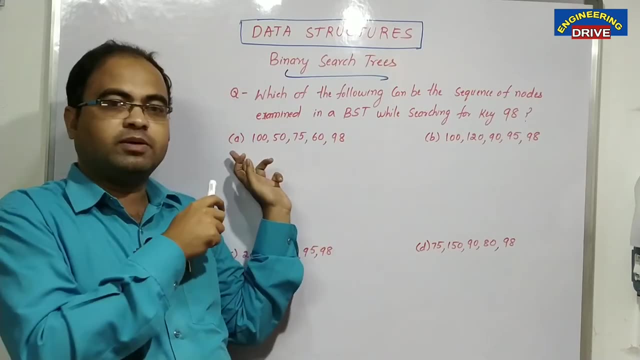 a node that is 98. So how I can travel the tree, How I can travel my binary search tree, Okay, whether sequence number 8,, whether sequence number 9, whether sequence number 10, whether sequence number 8 is correct, whether this sequence is correct, whether C is correct or whether D is correct. So, 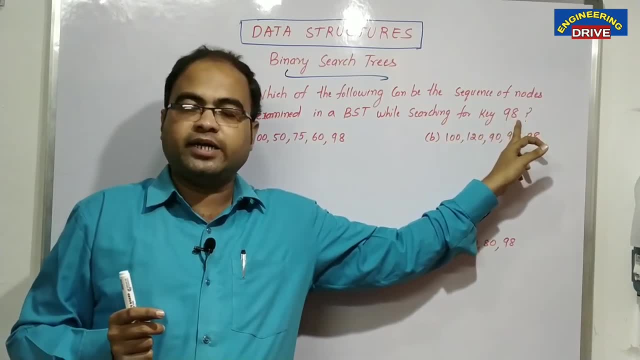 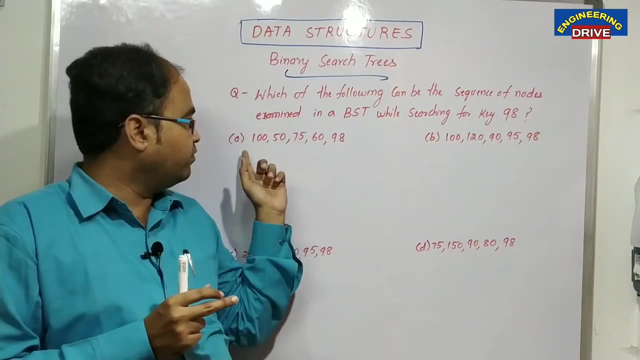 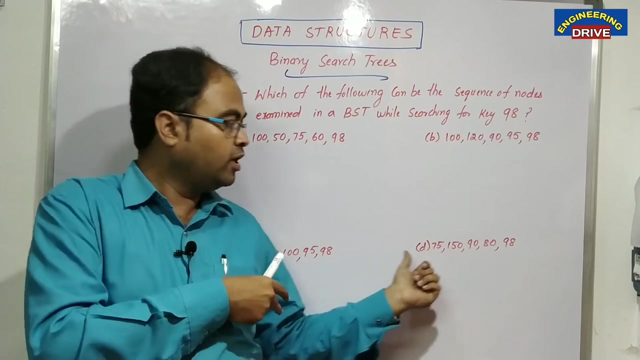 the simple question is: you need to search the value 98.. If you want to search the value 98, how you are going to visit the nodes. This is the question So, whether you will visit in this way, whether you will visit the option B, whether you will visit the nodes related to option C or whether 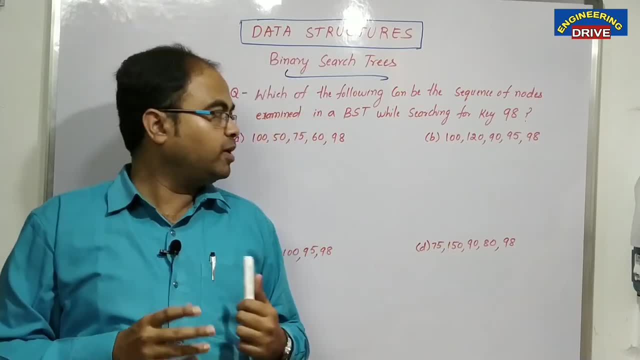 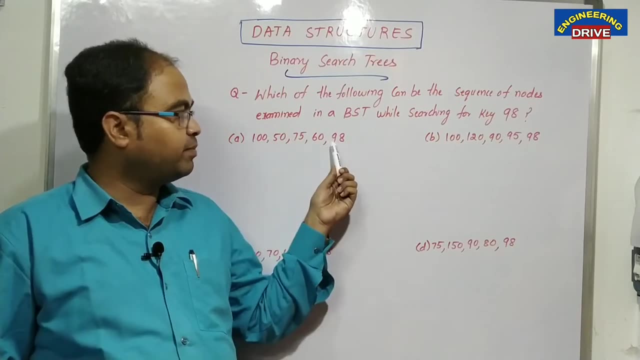 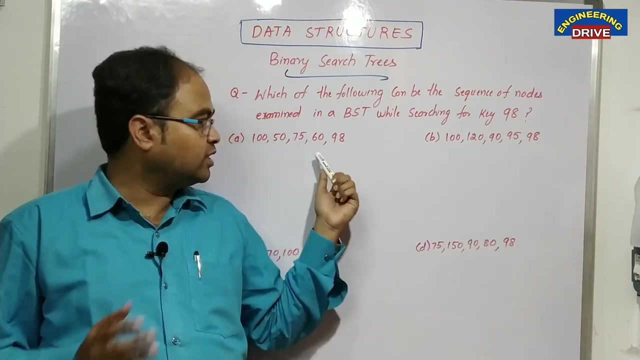 you will visit the nodes related to option D, So many people they don't know and they will face up to the answer in a wrong way And many people will get confused by seeing this number 98.. 98 is available last in all the options, So you can't say that B is the correct or D is correct, because 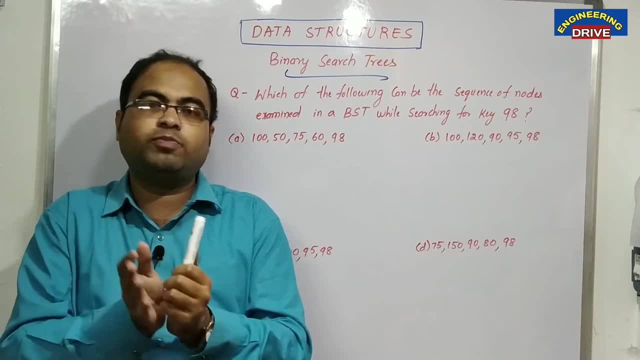 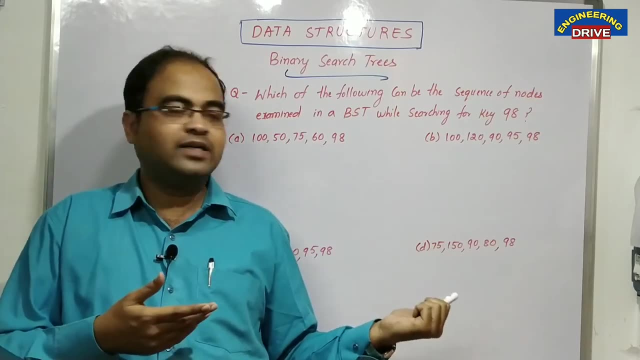 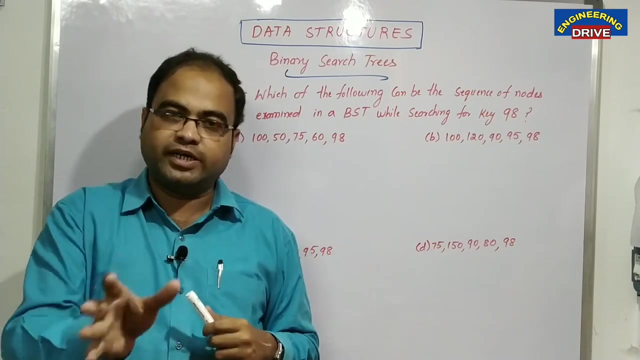 we need to search. 98 means that should be our ending point. But to confuse us, in all the options we got 98 last, So we can't guess now which one is correct. So how to solve this type of answers? It is very simple. You need to know the binary search tree conditions first, which we 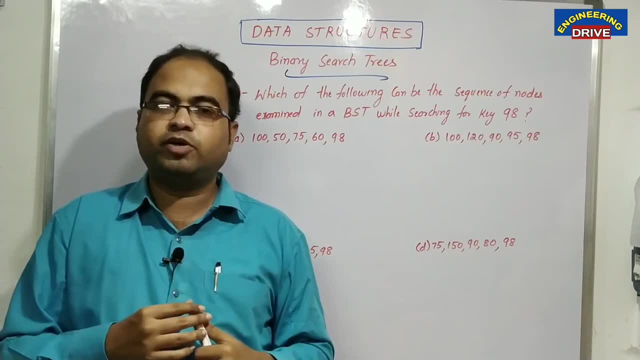 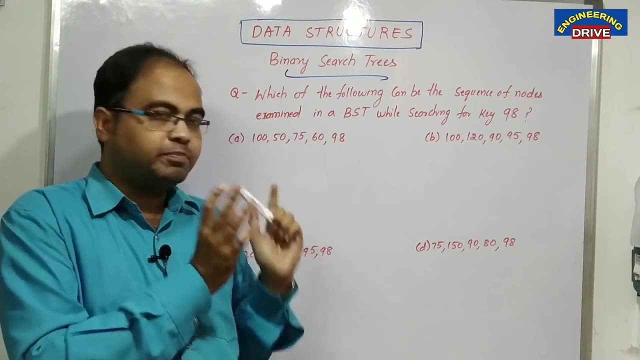 discussed now, which we already discussed now at the start of our today's video. Now you simply need to take one-one option. You need to construct the trees, That's all. You need to construct binary search tree for every option, Then you can get the correct answer. So how to construct a binary. 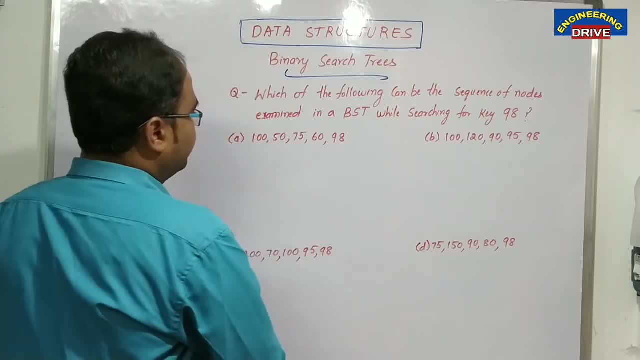 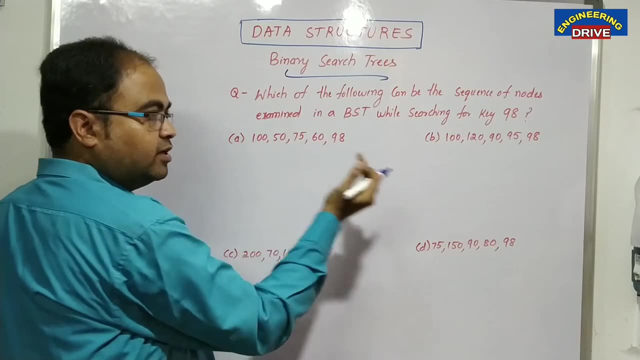 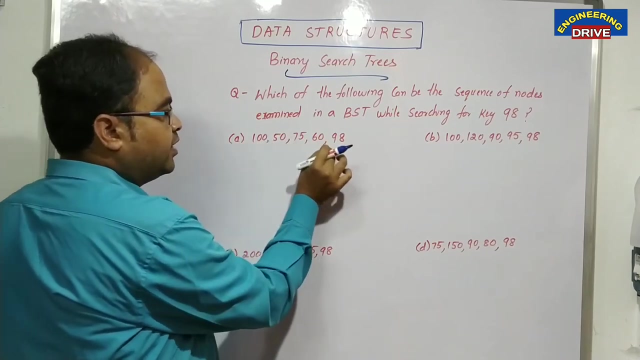 search tree. now, See here, let us take the option number A first. So which is the first value in the option number A? Now you need to travel the binary search tree Just now. previously I told you that the first node, always in any order or any sequence of orders of nodes, is always a root. 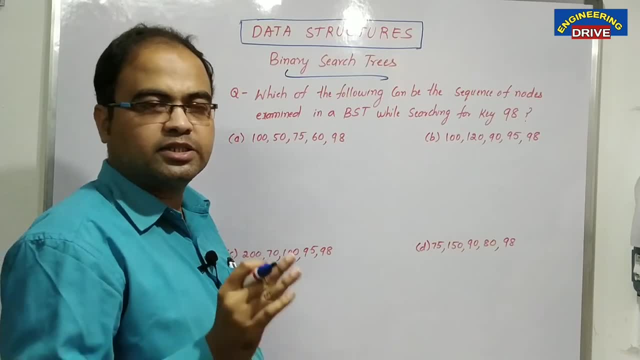 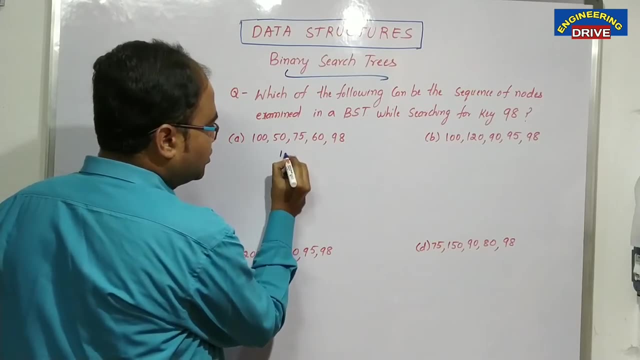 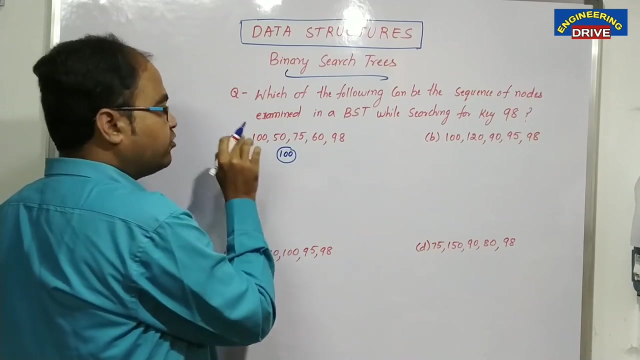 You know, a tree construction or a binary search tree construction always start from top to bottom, which means which node is available at the top? always root node is available at the top, So write down the root node. So why have taken 100? only root node, Always the first number in the 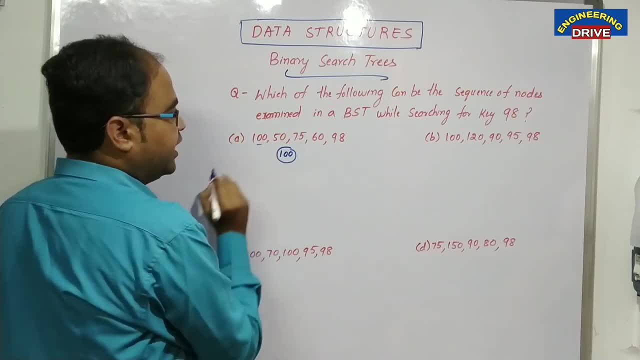 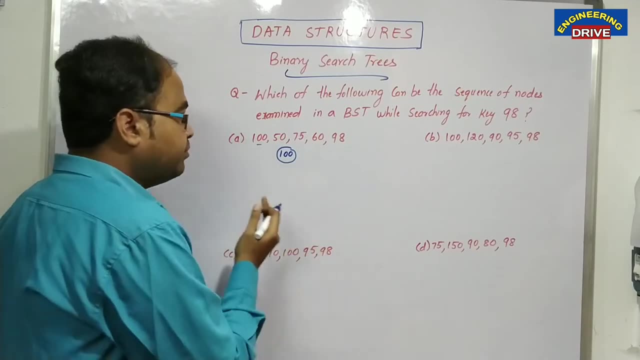 list 100. I have written Okay, So this number completed Second number 50.. 50 is less than 100 or it is greater than 100?. 50 is less than 100. Something which is less than the parent should. 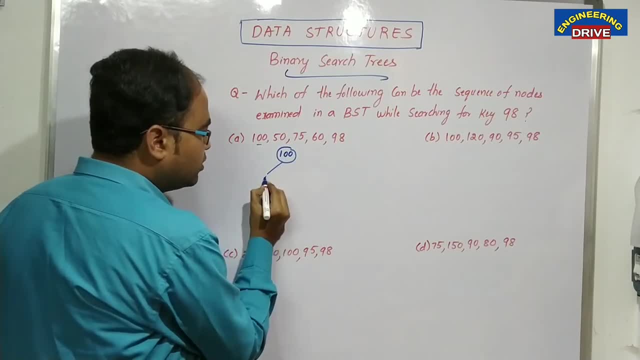 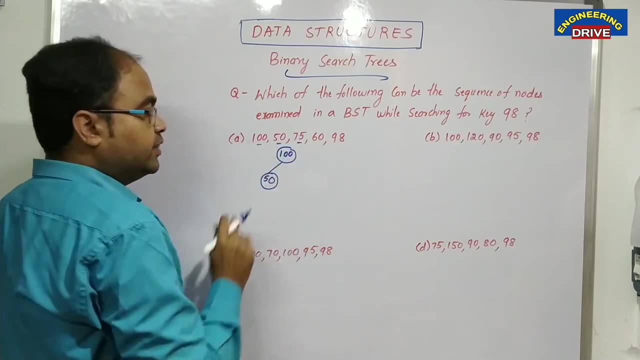 come on left side or right side. Of course it should come on left side. Very good, 50.. 50 completed. Next, 75.. Now 75. When you take the number 75, you need to see whether this number 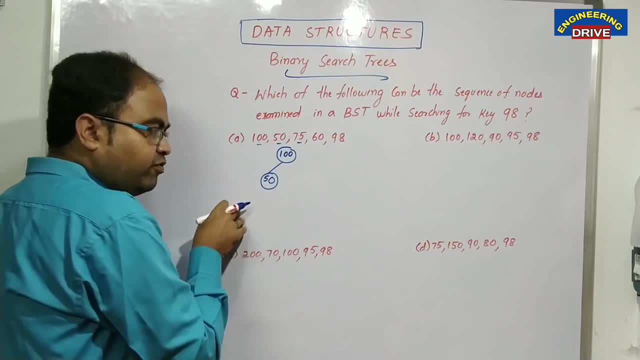 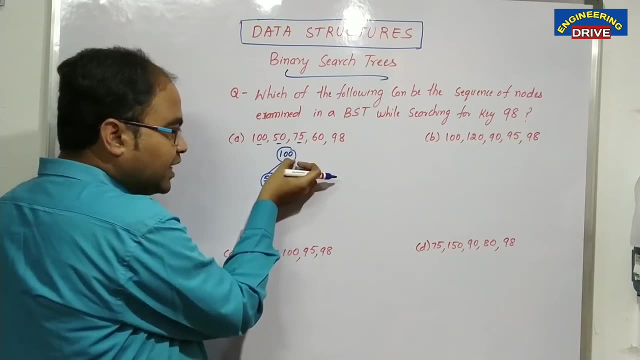 is less than 50 or greater than 50. Okay, You can see here. First check the root node now first Whether this 75 is less than 100 or greater than 100? Less than 100. So it will come to left side. 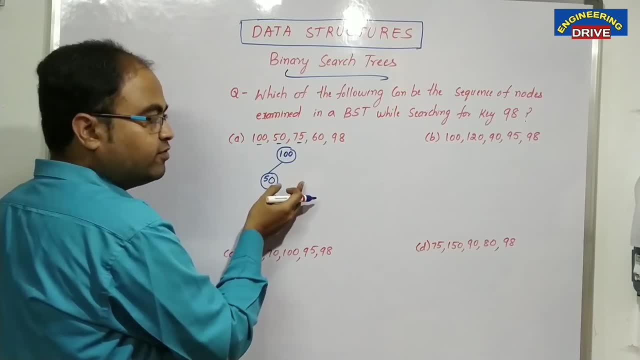 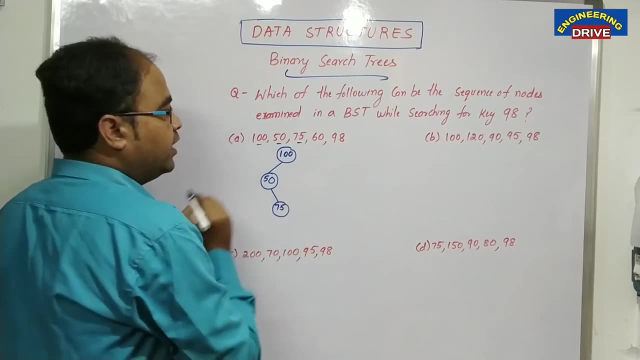 Now check 50.. 75 is less than 50 or greater than 50? Greater than 50. Greater than means it will come on right side, So this is 75. Okay. Next take the number 60. Okay, 60 is less than 100 or. 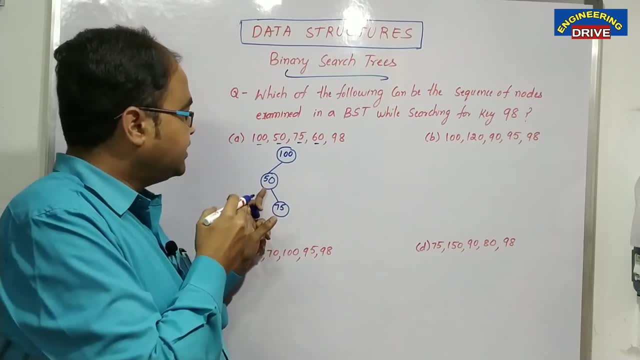 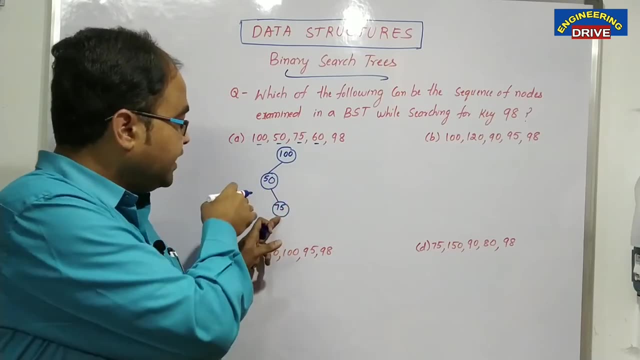 greater than 100? Less than Come to the left side. 60 is less than 50, or greater than 50? Greater than 50. Come to the right side. Come to the right side Now. 60 is less than 75, or. 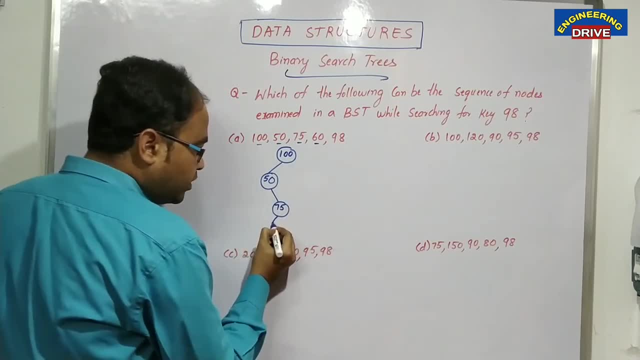 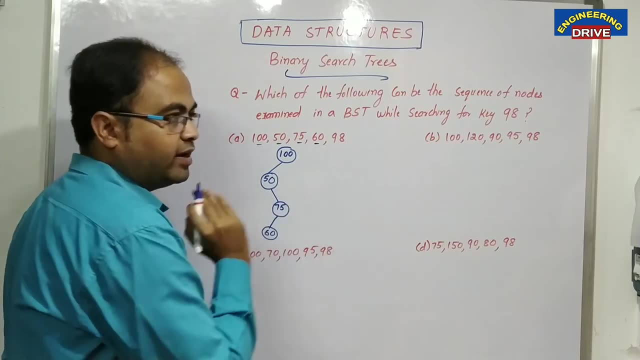 greater than 75? Less than 75.. So where I should write this one, You should write here 60.. My dear students, where to write left sides or how to write right side, Many people will get confused here. So something which is less than the parent always come left, Something which is 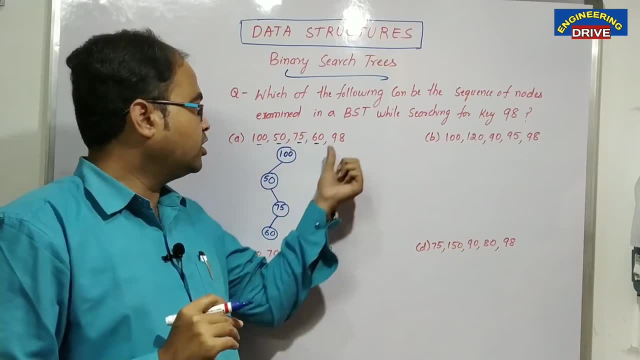 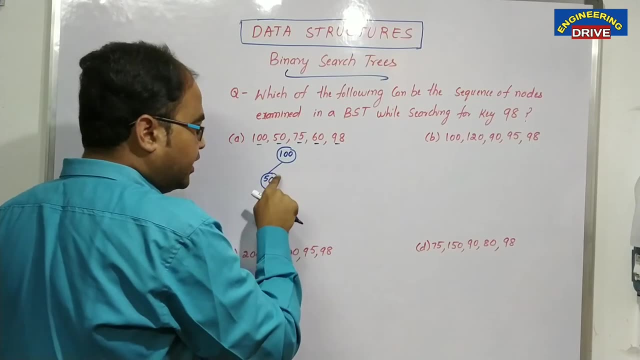 greater than the parent always come left. Something which is greater than the parent always comes on the right side. Okay, Now, what is the last number now here, in our case, 98.. 98 is less than 100 or greater than 100?? Less than So, it will come here. 98 is greater than 50, or 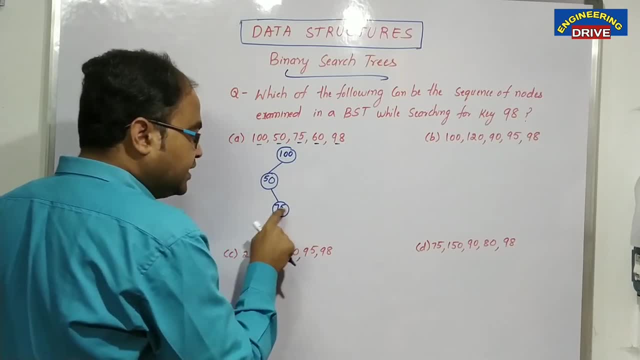 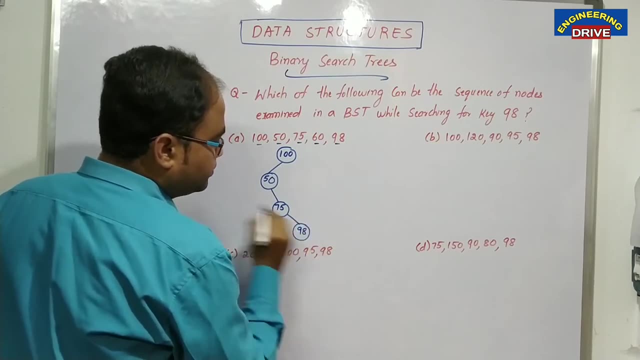 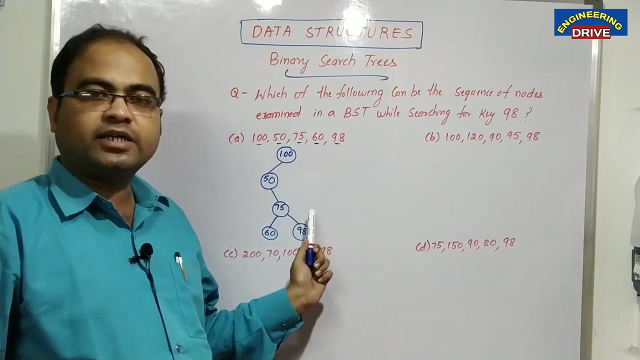 less than 50? Greater than 50. It will come here: 98 is less than 75 or greater than 75? Greater than 75, which means you need to write here 98.. Okay, Whether this answer is correct to search the key 98?. No, it is not the correct answer because, finally, 60 and 98,. 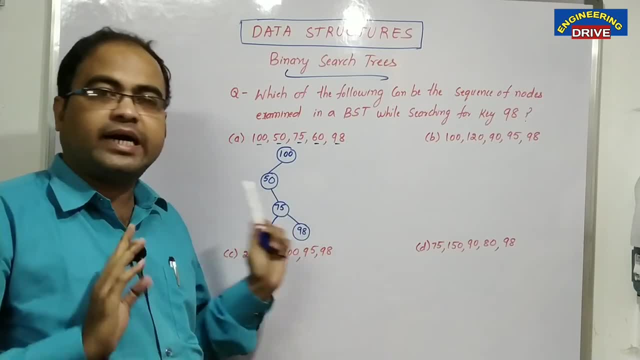 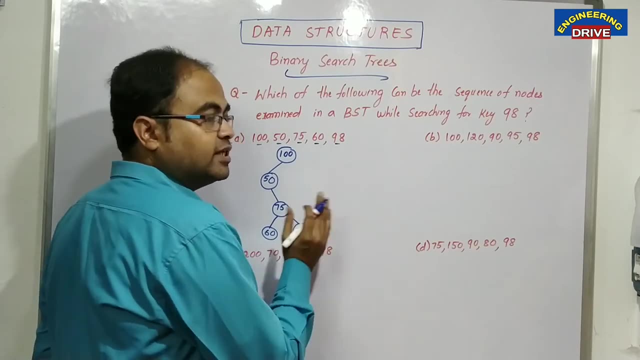 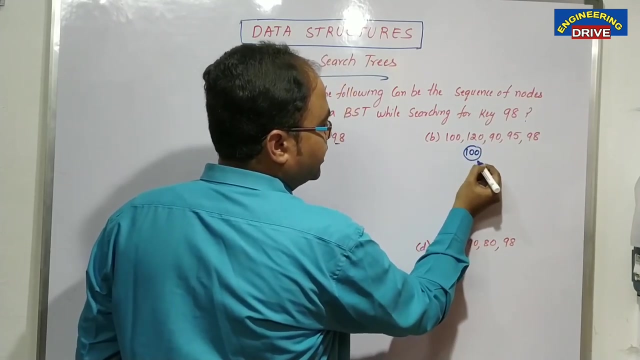 they are child for same parent: 75.. So this is not our correct answer now. So let us verify the second option now. We need to search all these options now, Then we can know which answer is correct: 100.. So take always: 100 is the root. note 120.. Less than or greater than greater than 100?. 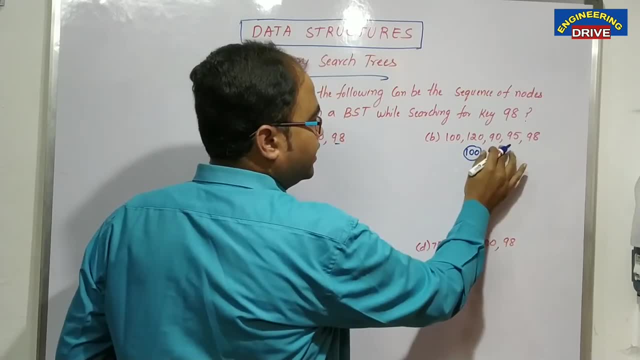 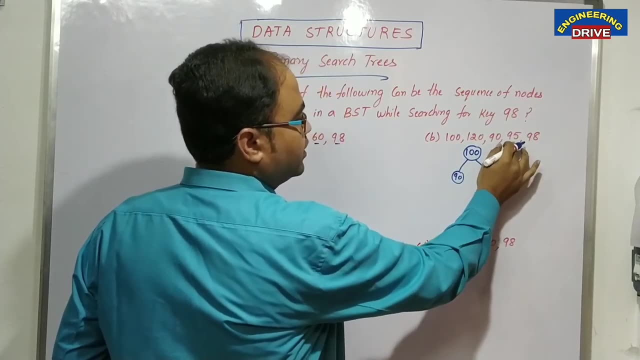 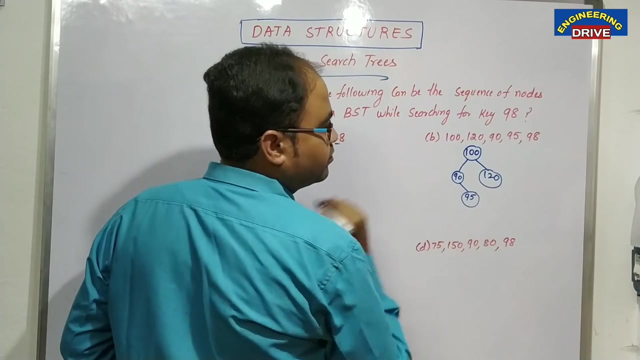 It will come on right side. Okay, 90. 90 is less than 100.. So which means it will come here 90.. Next 95.. 95 means less than 100. So it will come here. It is greater than 90. So you should write here: 95. 98. So 98 means less than. 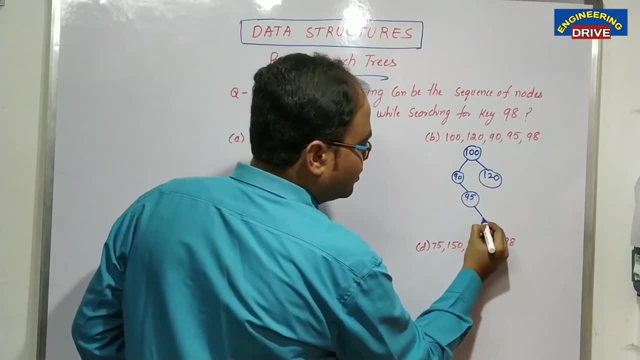 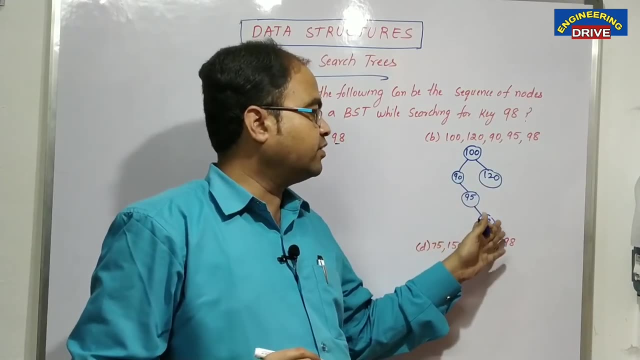 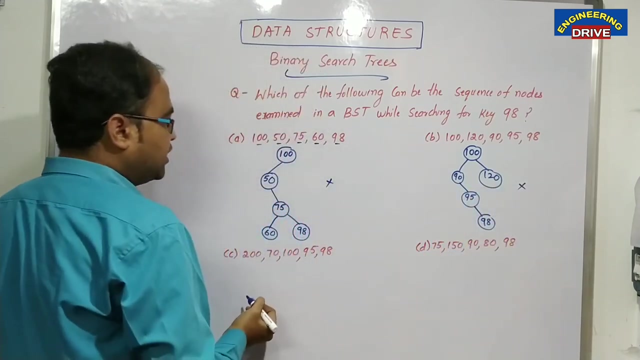 100.. It is greater than 90 and it is greater than 95. So, of course, this is also not the correct way of visiting and searching for key 98.. Okay, So we did not get the first option and we did not get the second option also. Let us see the option. 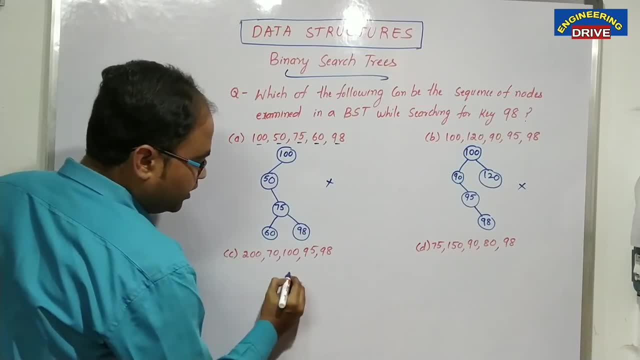 number 3. now, Okay, So first, which is the root note here? Here we got the root note 200.. Next, 70. It is a less value. That is why I am writing on the left side: Next, 100.. 100 means less than. 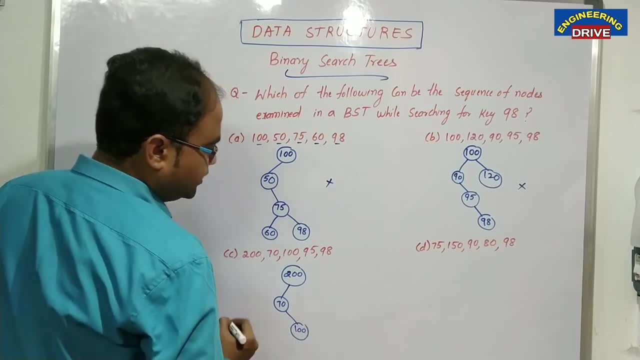 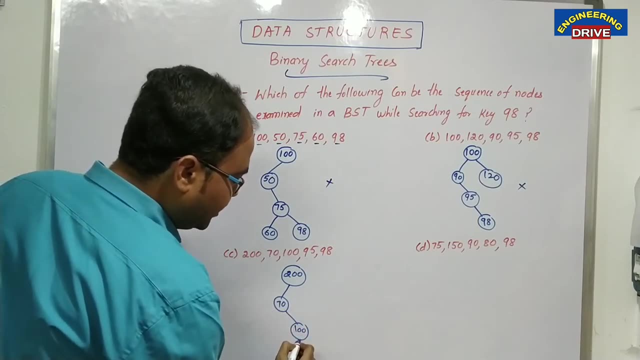 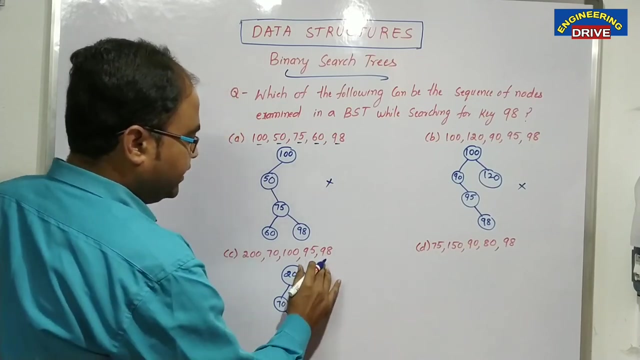 200, but it is greater than 70. So, right side, 95.. 95 is less than 200, but it is greater than 70.. Where I should write this 95? It is less than 100 or it is greater than 100, less than So here I am writing 95.. 98.. 98 is less. 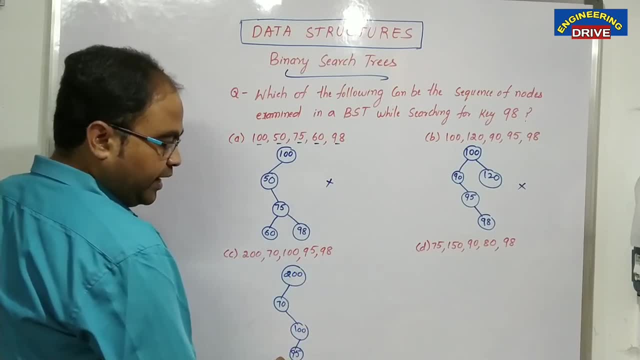 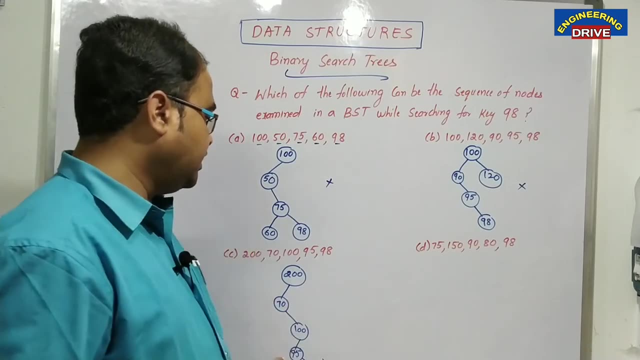 than 100.. Yes or no, But 98 is greater than 95.. So where I should write Here: Okay, Now when we see, you can see that from 200, we have visited to 70.. From 70, we have visited to 100.. From 100,. 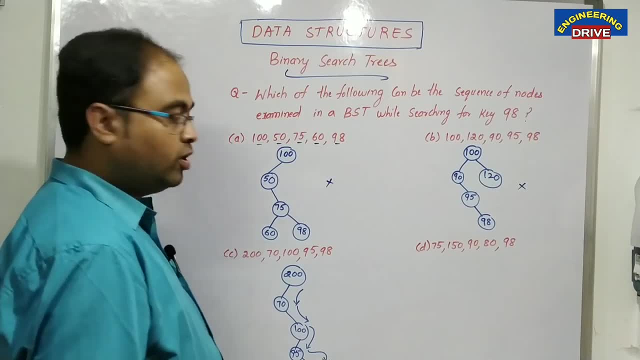 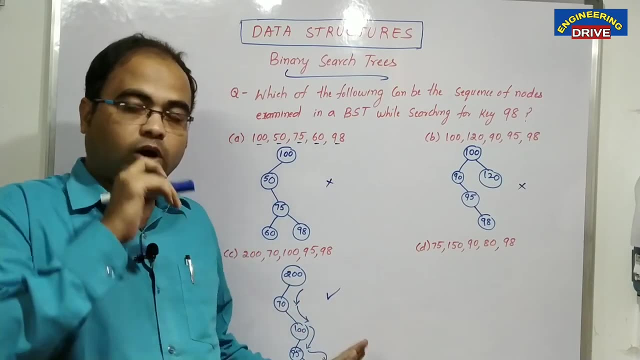 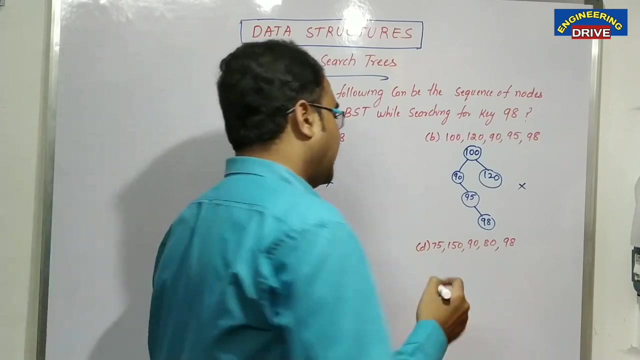 we have visited to 95. 95,. finally we have visited to 98. So option number 3 is our answer. So finally, we have visited and we have got that key 98 at the last. That is why option 3 is our correct answer. If you want, you can verify the last.